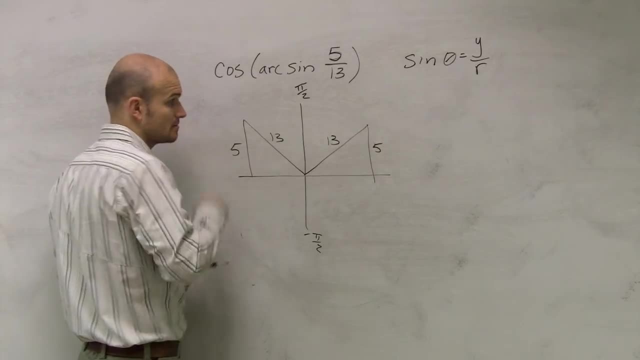 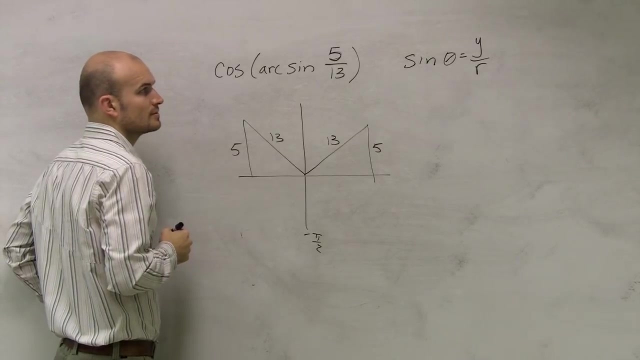 Right. So therefore, yes, How do you know which ones are the hypotenuse Like? because it's arc sine Like. how did you know 13 was the hypotenuse? You just say sine, is that? Well, remember, r represents our hypotenuse. 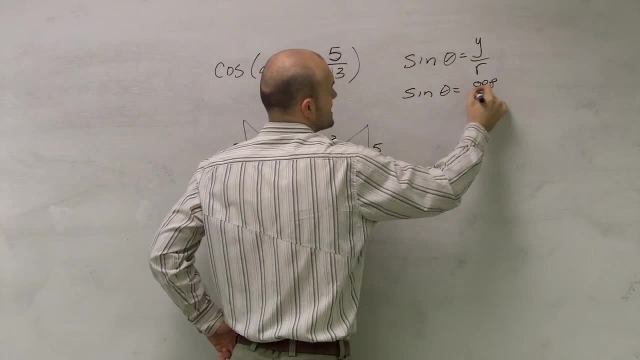 Or if you want to go back a little bit to other training, you can also do. remember it's always the opposite over hypotenuse. So you just substitute sine for cosine or arc sine. No well, I haven't finished it yet. 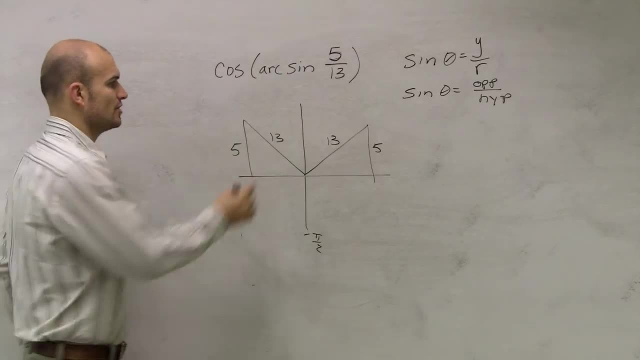 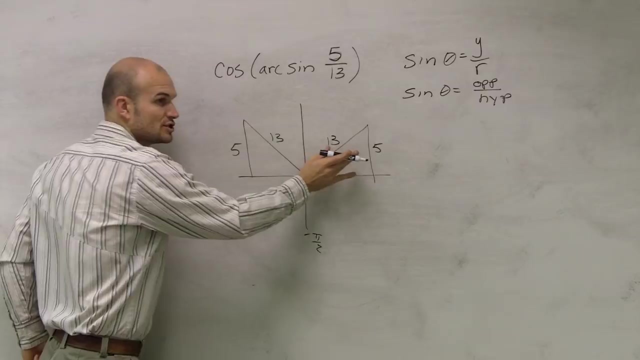 But just finding the inverse. I'm going to use my inverse sine to go ahead and determine what my triangle is. So the reason why we have the inverse sine is giving us a restriction that we have to only use this triangle because that is within our constraints. 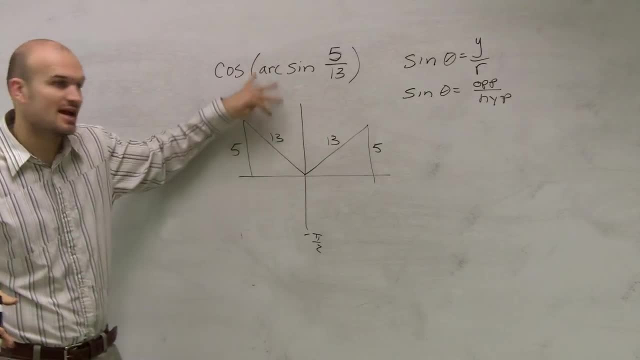 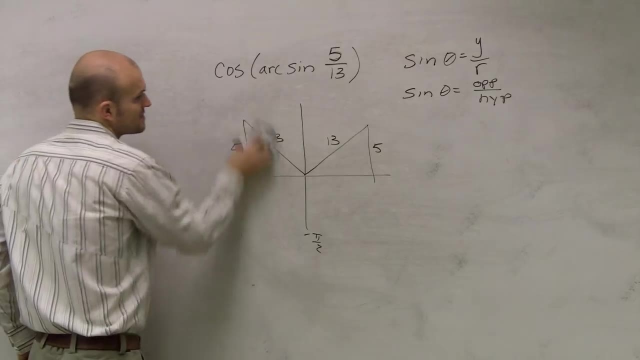 All right. So that's why we use the inverse sine, And so I can say: hey, I can't use this triangle, Otherwise we'd have two answers, right? We wouldn't know which one to pick. So since I'm using inverse sine, I'm going to be able to eliminate this triangle. 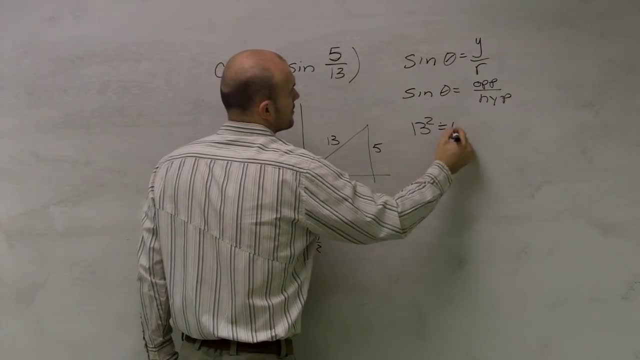 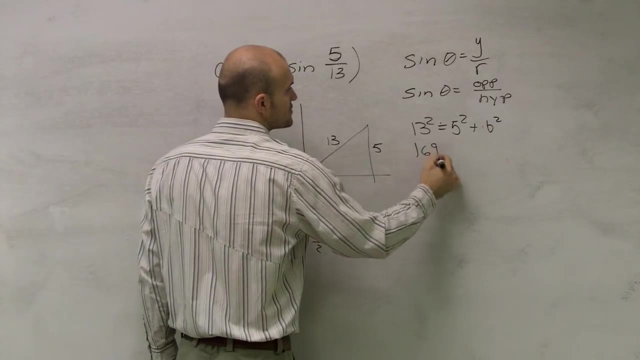 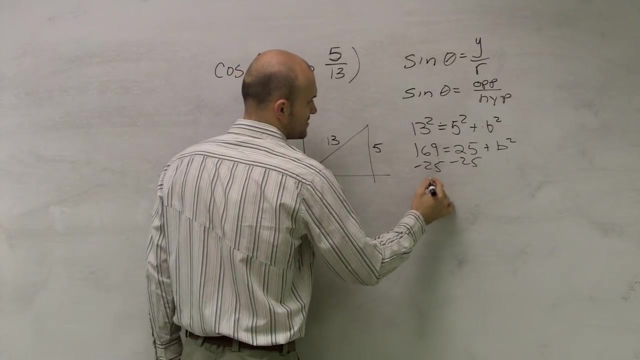 And I can use now Pythagorean theorem to solve for this. So I have 13 squared, which is 169, equals 25, plus b squared minus 25.. Yeah, I know it's going to be 12 squared. 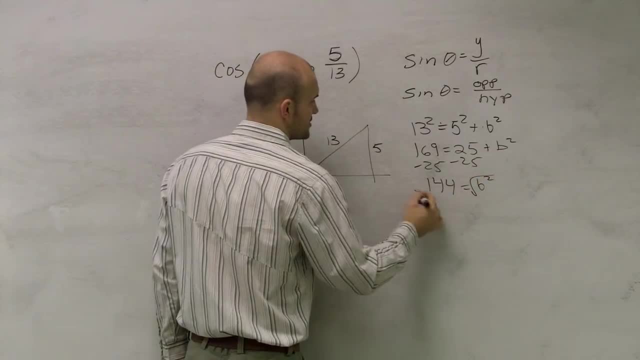 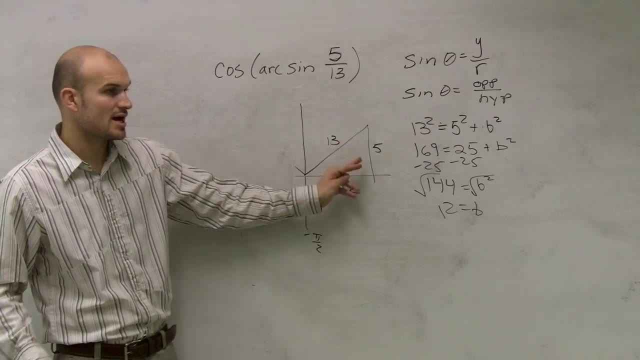 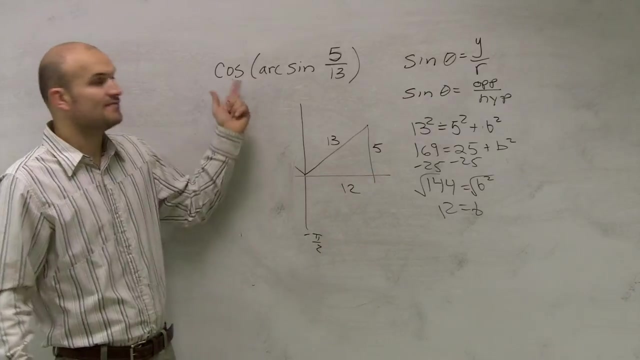 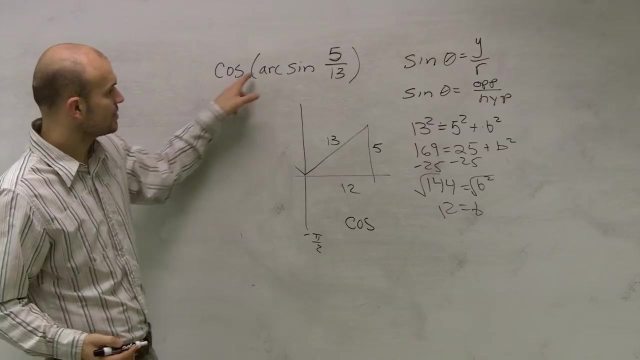 But I'm just going to show the work just so I don't make sure everybody understands. So therefore I have my triangle, Now I've determined what my angle is for my x value. So then it says: find the cosine of this. Well, cosine of your angle, cosine of this is going to be your adjacent over your hypotenuse, or your x over your r. 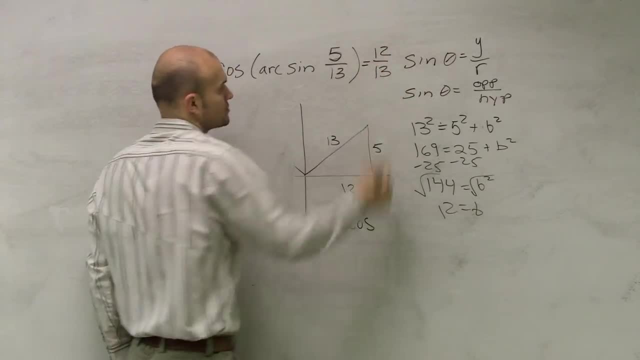 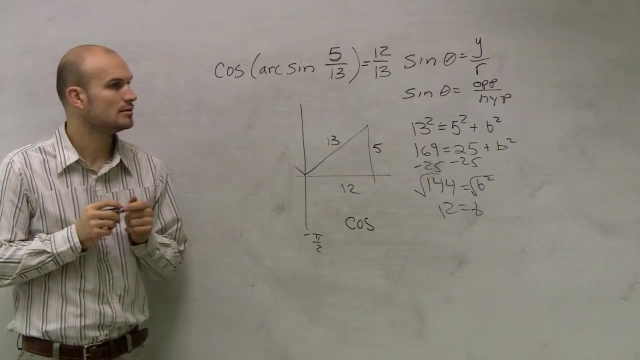 So the final value for this is just going to be 12 over 13.. Make sense, Tamara. you had a question, Yeah, how she asked earlier about how you know which one's the hypotenuse and everything. how do you do that? 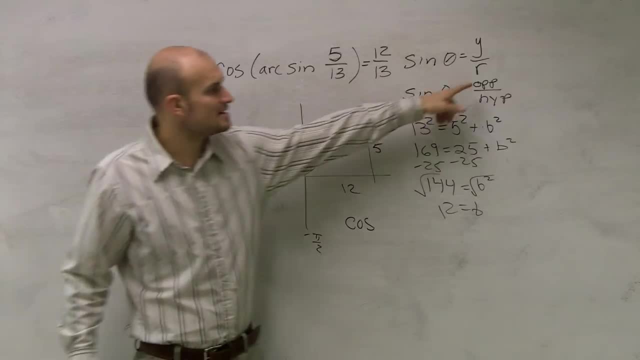 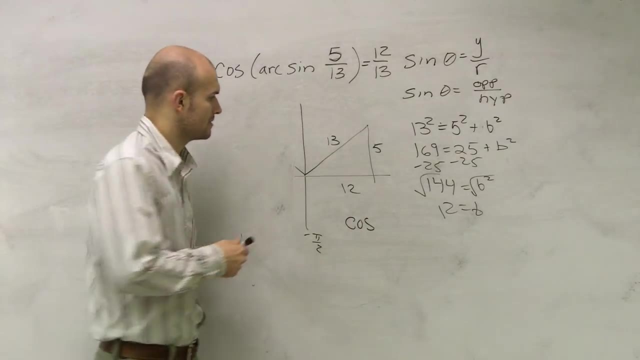 Just remember that when you're dealing with sine, that is your opposite over your hypotenuse. If you're dealing with cosine, remember cosine was your adjacent over your hypotenuse And I mean we're just going to be working.